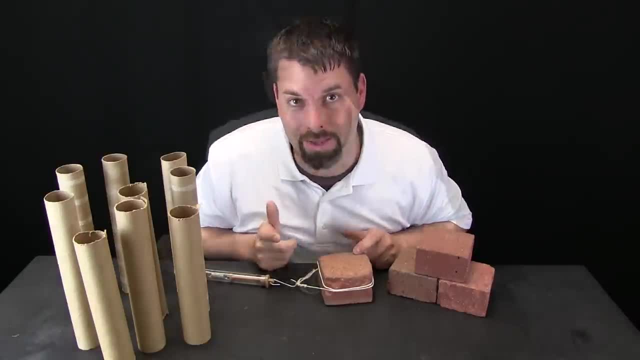 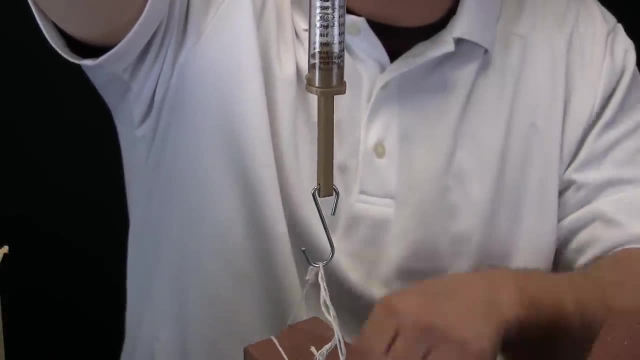 So let us start with a question: How much does this brick weigh? To figure that out, we are going to use our spring scale. So take a look at this. I am going to lift the brick off the table and take a look at our spring scale. It is reading a little. 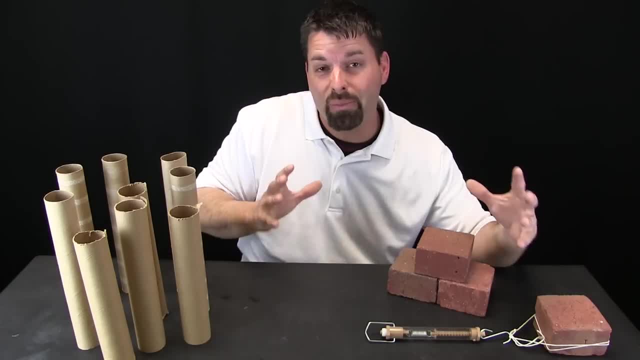 over a hundred centimeters. It is a little over a hundred centimeters. It is a little over a hundred centimeters. It is a little over a thousand grams or right out of a thousand grams. Now those big blocks of stones in the real Great Pyramids weigh a lot more. There is no way they 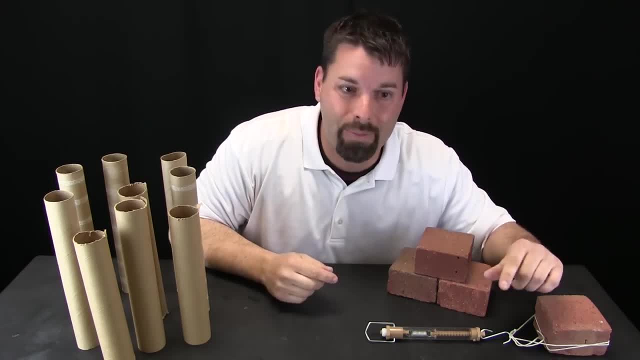 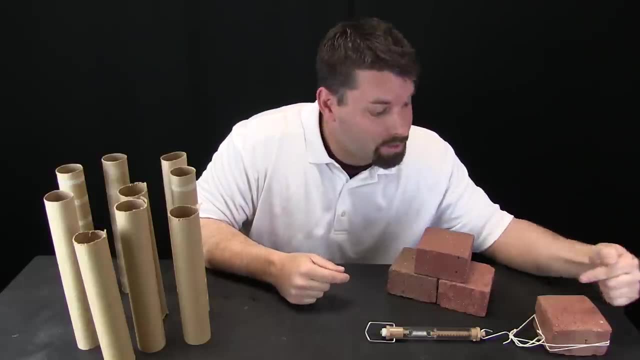 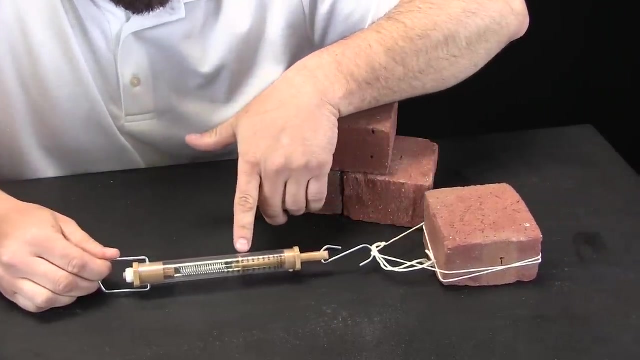 could lift those blocks up and carry them. So let us see what happens if we try and drag this brick, If they could drag those big blocks of stone and see how many grams it takes to move this brick if I drag it. So now let us try dragging our brick. I get it started moving and I can look It is. 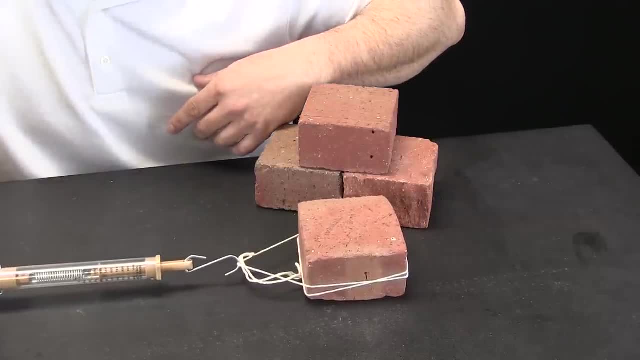 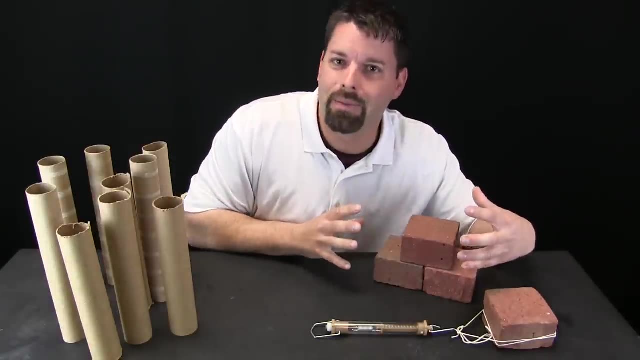 between three hundred and four hundred grams as I drag the brick. So it was easier to drag this brick than it was to lift it up and carry it. But the blocks that made up the Great Pyramid were so big and so heavy that they were even really difficult to drag. So 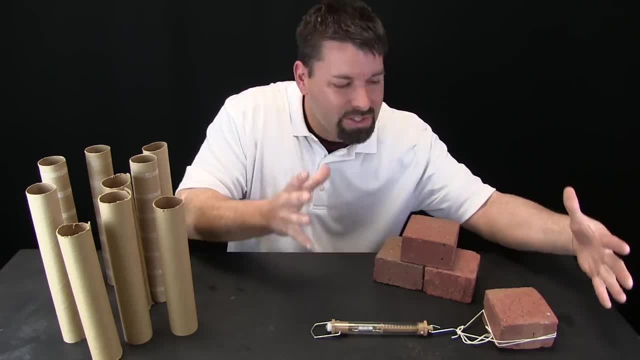 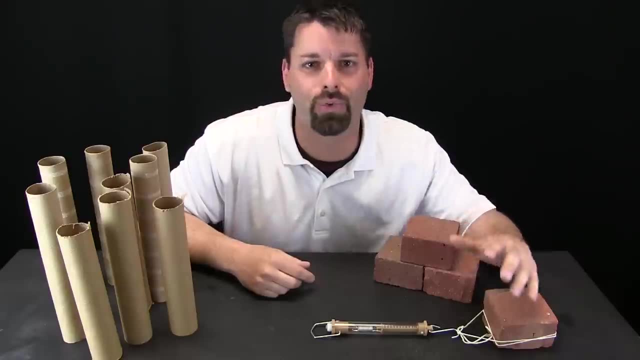 the people back in history had a problem: How do we move these massive, huge, big blocks of stone? Well, through science, we have discovered that you usually solve problems by asking the right questions. What if? What if I cut these trees down and use these rounds? 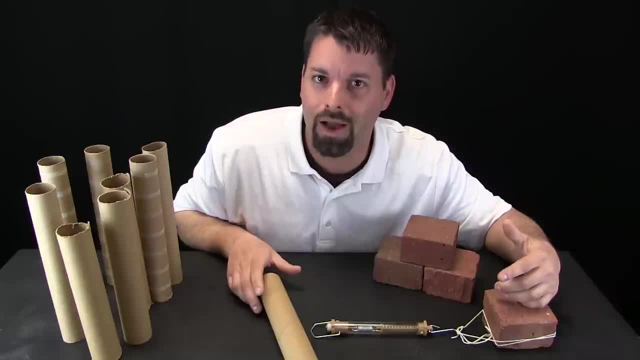 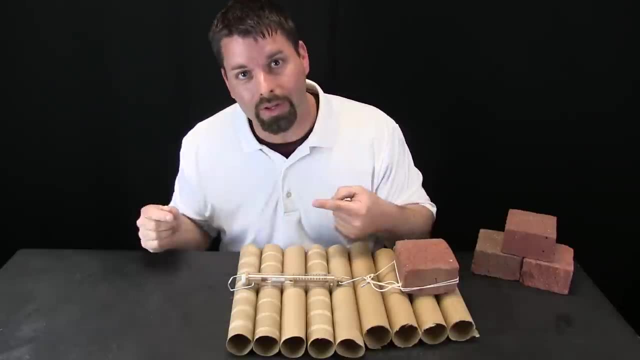 these round logs to go under the block. I wonder if that is going to make our work easy. So we have placed our block on top of these round tree logs and now we are going to pull it and see if our work is easier. 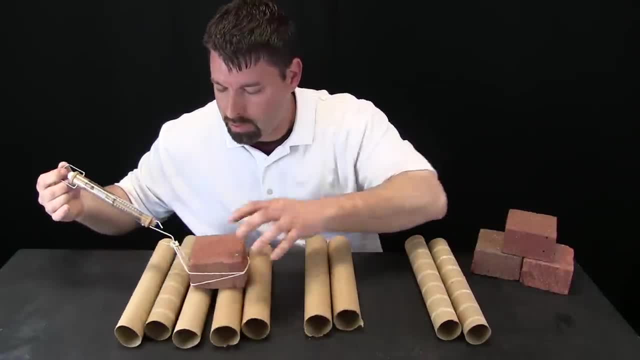 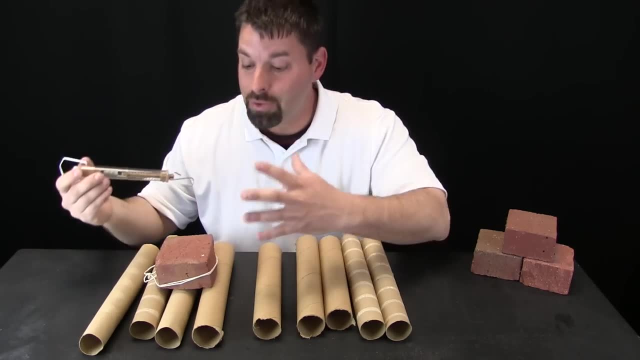 Let us try it out. So I gently pull. Believe it or not, my spring scale barely moved off of zero grams. It hardly took any energy to move this block on these round tree logs. But what do we do now? We are out of tree logs. 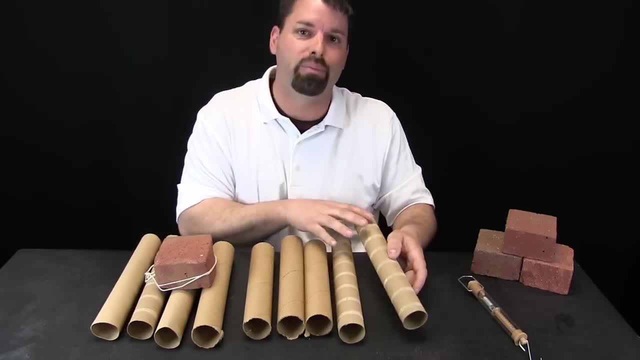 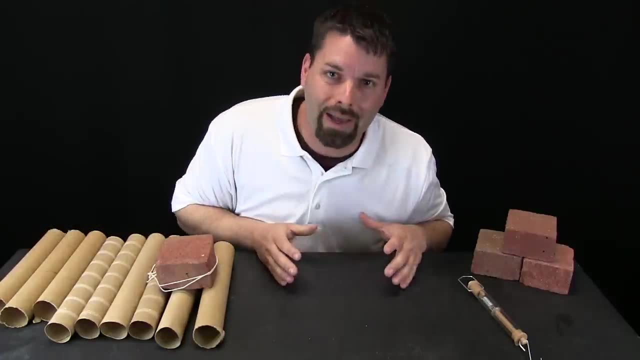 So that means we would have to pick up this tree log and move it to the front. pick up this tree log and move it to the front. pick up this tree log and keep moving the tree logs to the front from the back. Well, that is a lot of work too. Well, good news, Science is not finished yet. 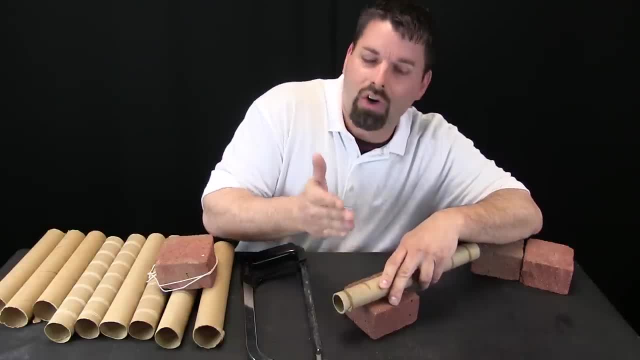 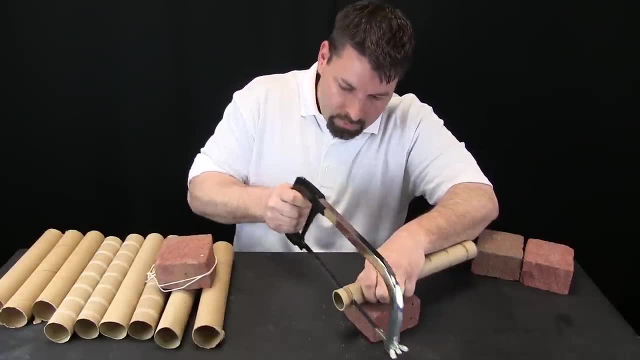 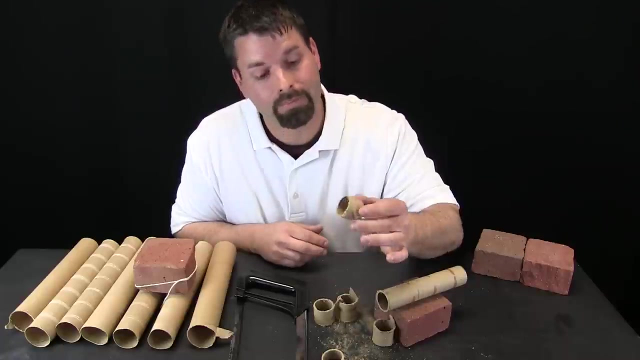 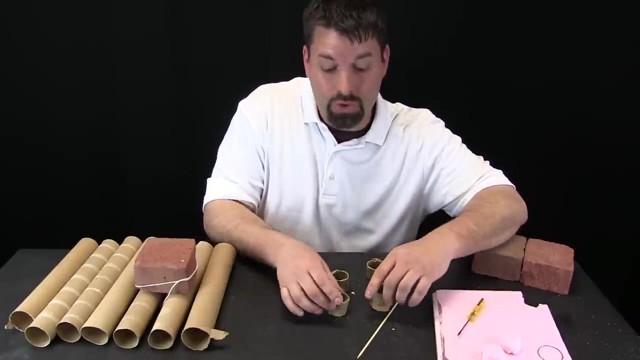 Well, what if I take this tree log and cut sections off of the tree log? Let us see what we are left with when we do that. So what have we got? Well, we have the wheel, But how do I attach this wheel to our block? Well, through science, we have discovered that we can attach邗 wheels with an axle. 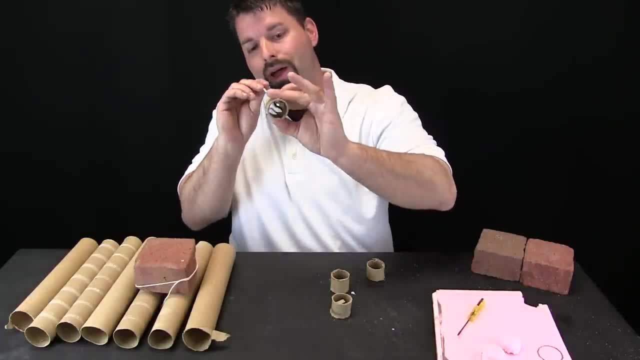 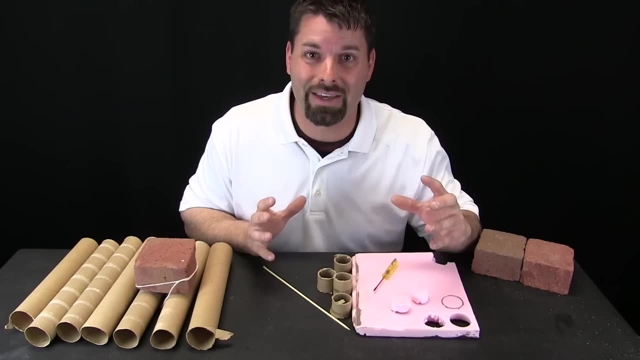 This piece of wood is going to be our axle, but I need some way to attach the axle to the wheel, And to do that I am going to use styrofoam. Now, cutting styrofoam is really not a kid-friendly thing to do. It is difficult and you do not want kids using sharp knives or cutters. So we came up with a code for quirks in apes and beastles. So we are going to get our styrofoam cut into the head position, whereas we are going to use a sh skyward cutter. In that case, we are going to cut it decorationally. Now can we try and get the off. Now can we get the off. 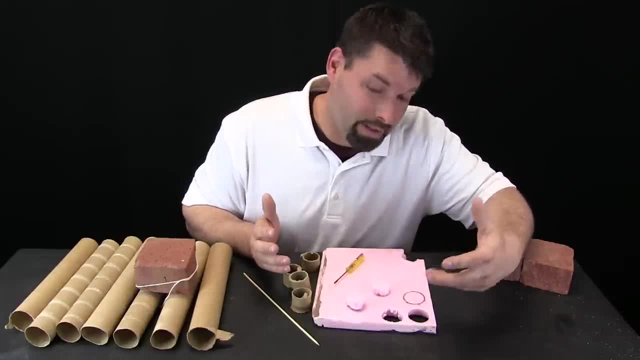 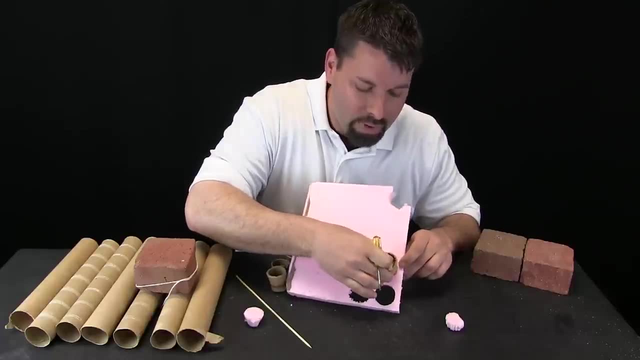 Yes, Yes, Yes, And we came up with a really kid-friendly way to allow kids to cut Styrofoam. It may not be the prettiest, but it works. So all I am going to do is trace my wheel on my Styrofoam and use something thin like. 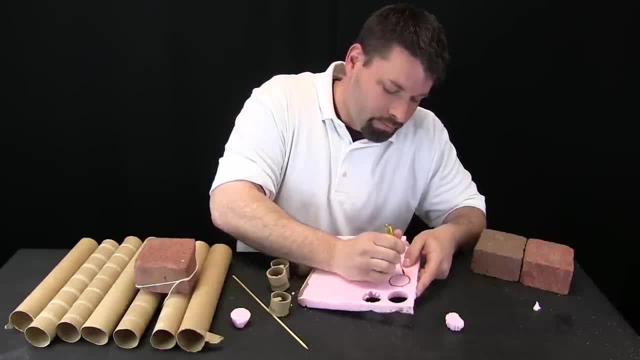 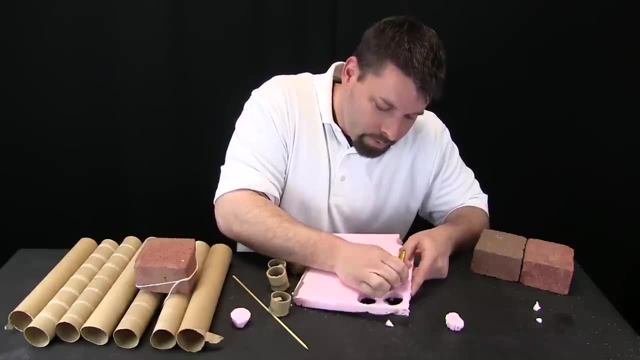 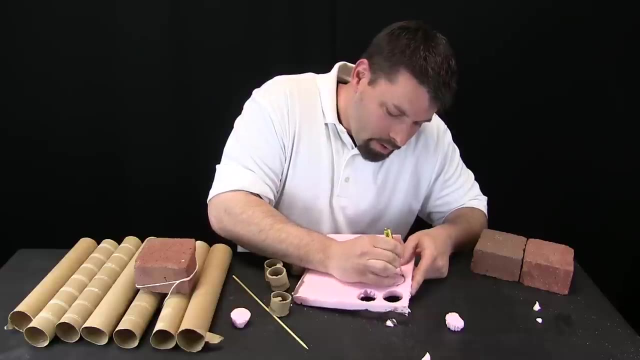 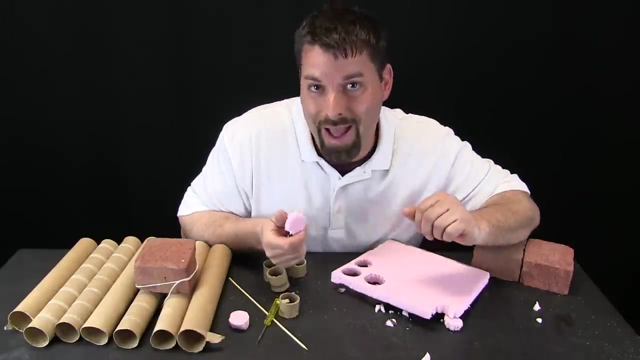 this screwdriver and just go around the wheel punching down the Styrofoam, taking my time working my way around the wheel. It is pretty easy to push through the Styrofoam And once I get all the way around now all I need to do is push and it comes right out. 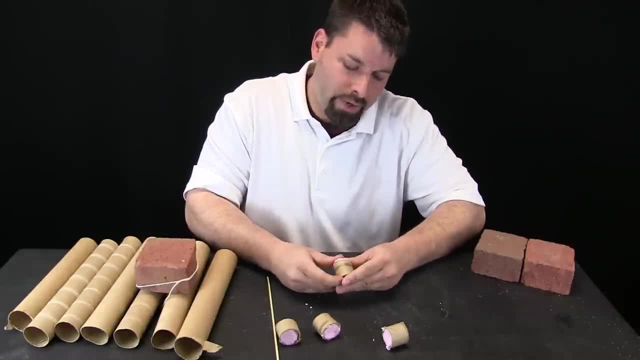 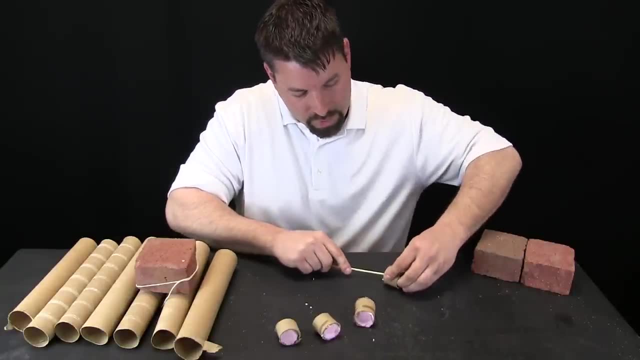 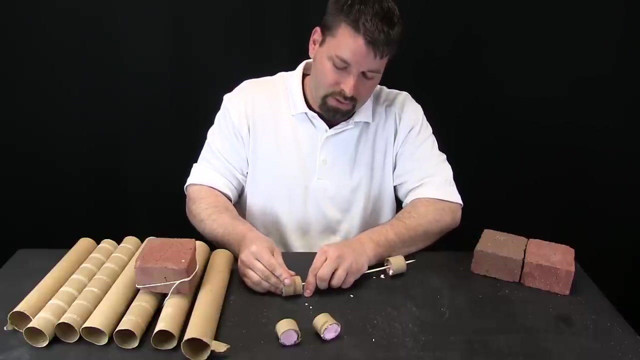 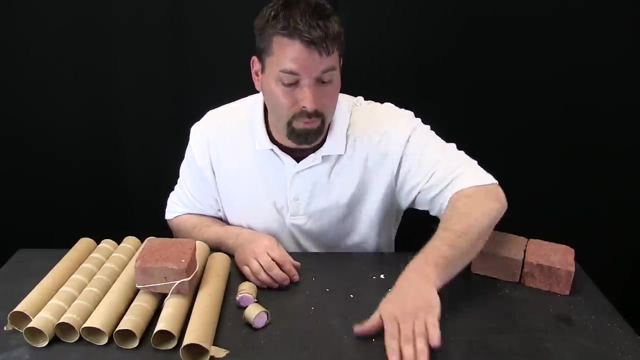 Now we need to take our Styrofoam plug, put it into our wheel and now I am ready to attach my axle. Just going to push my axle into the Styrofoam- The Styrofoam on both sides- It looks like I have a wheel base that is ready to roll. 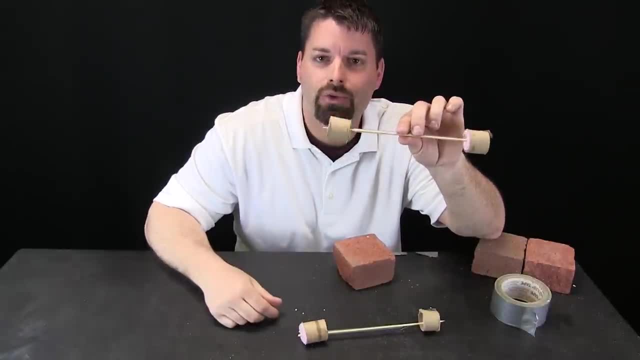 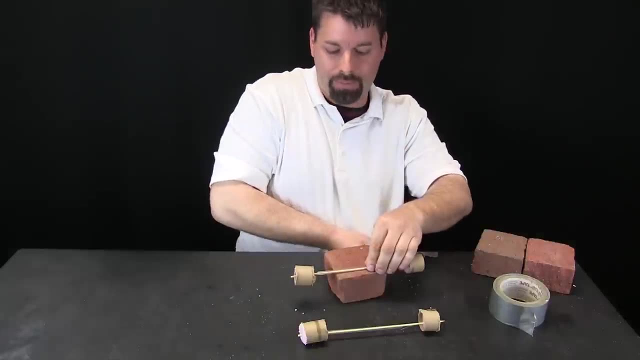 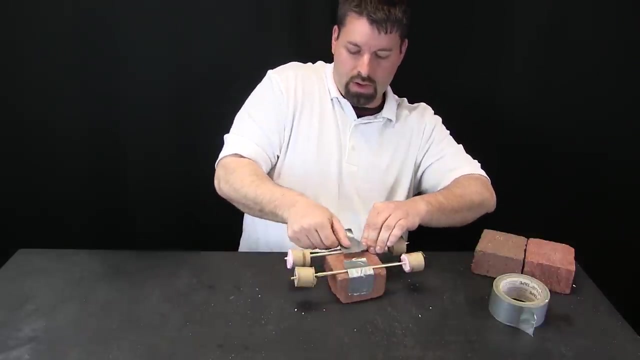 We also took a clear straw and put it through the wooden axle so our wheel and axle can spin quite easily. Now we have to attach this to our block and we are going to use some tape to do that. One piece there, One piece here.